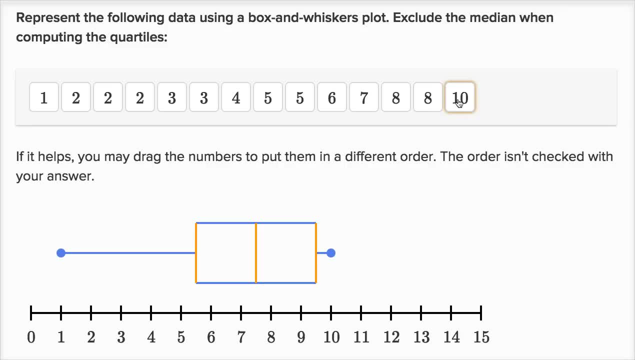 eleven, twelve, thirteen, fourteen numbers. Since I have an even number of numbers, the middle two numbers are going to help define my median, Because there's no one middle number. I might say this number right over here, this four, But notice there's one, two, three, four, five, six, seven above it. 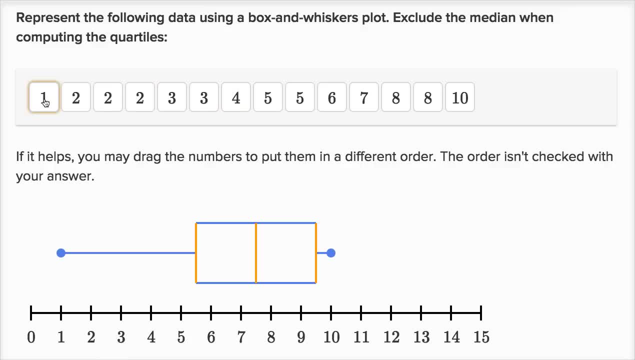 And there's only one, two, three, four, five, six below it. Same thing would have been true for this five. So this four and five, the middle is actually in between these two. So when you have an even number of numbers like this, 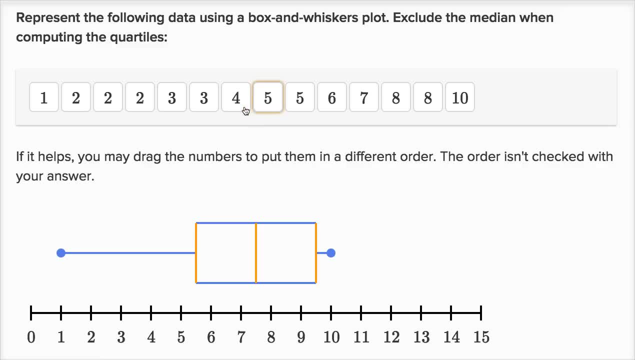 you take the middle two numbers- this four and this five- and you take the mean of the two. So the mean of four and five is going to be four and a half. So that's going to be the median of our entire data set. 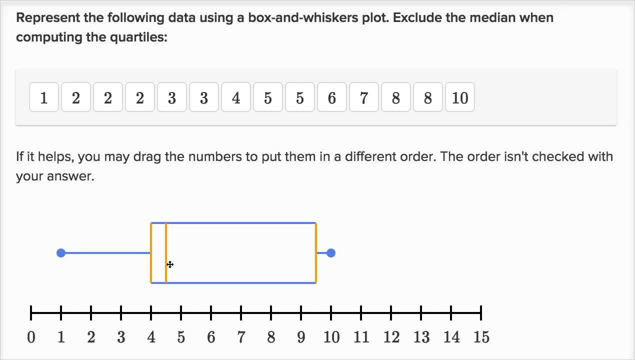 Four and a half, Four and a half, Four and a half. And now I want to figure out the median of the bottom half of numbers and the top half of numbers. And here they say: exclude the median. Of course I'm going to exclude the median. 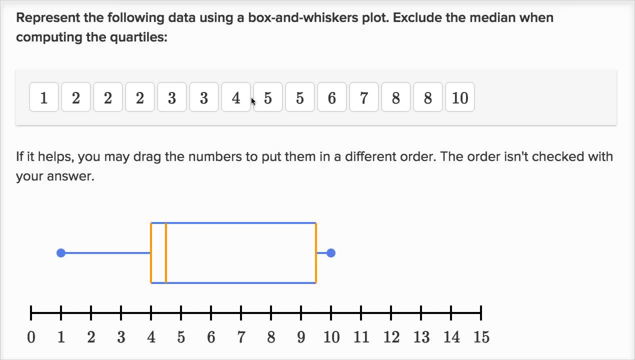 It's not even included in our data points right here, because our median is 4.5.. So now let's take this bottom half of numbers, Let's take this bottom half of numbers right over here and find the middle. So this is a bottom seven numbers. 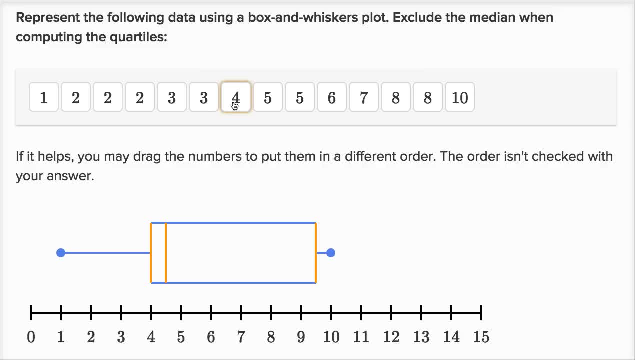 And so the median of those is going to be the one that has three on either side. So it's going to be this: two right over here, So that right over there is kind of the left boundary of our box, And then for the right boundary 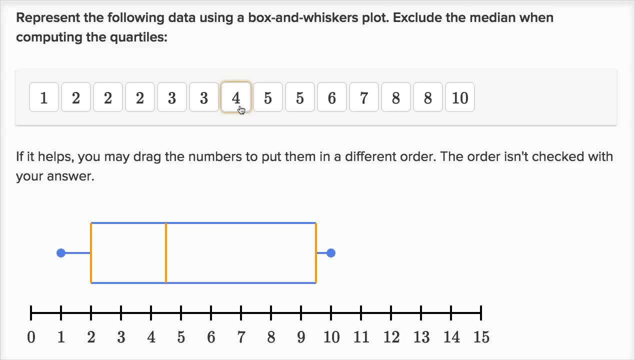 we need to figure out the middle of our top half of numbers. Remember four and five were our middle two numbers. Our median is right in between at four and a half. So our top half of numbers starts at this five and goes to this ten. 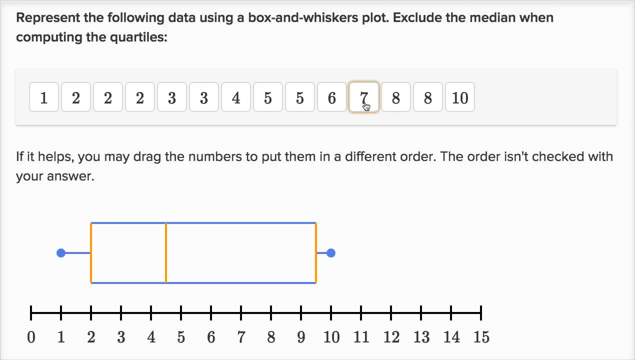 Seven numbers. The middle one is going to have three on both sides. The seven has three to the left, remember, of the top half, and three to the right, And so the seven is, I guess you could say, the right side of our box. 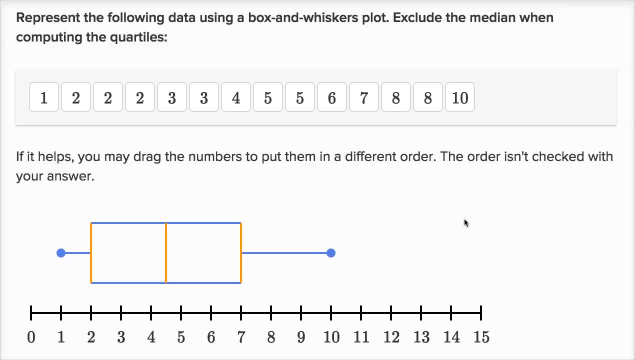 And we're done. We've constructed our box and whiskers plot which helps us visualize the entire range, but also, you could say, the middle, roughly the middle, half of our numbers.